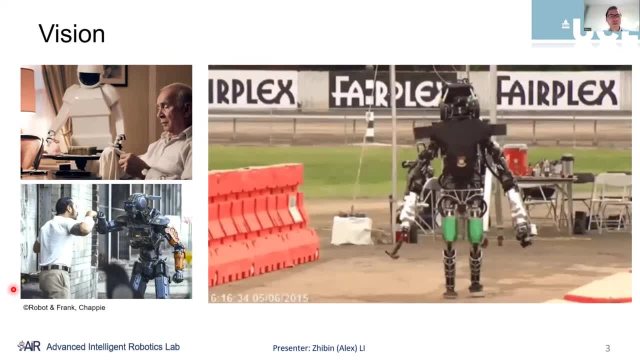 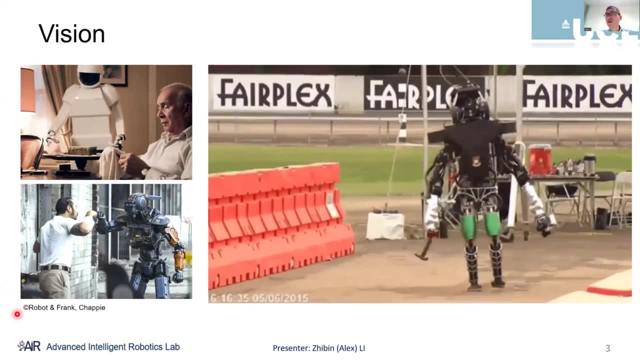 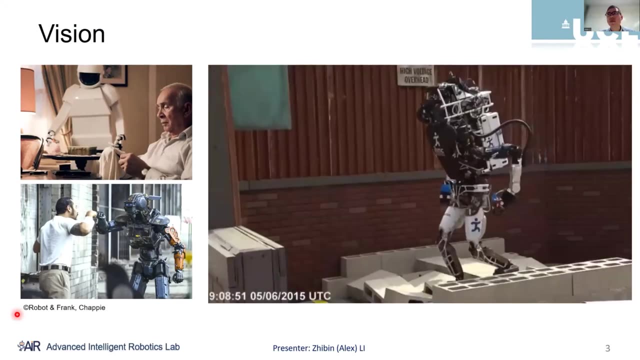 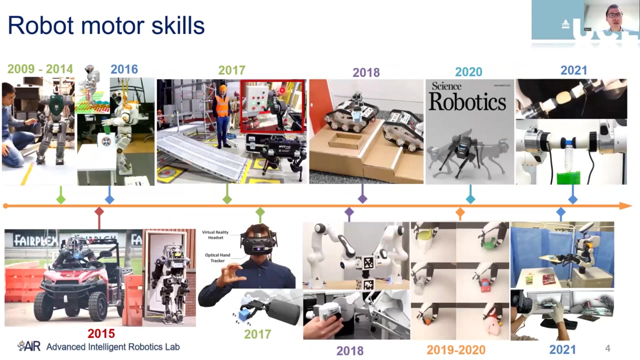 And personally for me, Because we don't have video, we don't have a screen, So, personally for me, the AI research is largely inspired by the DARPA Robotics Challenge And the robot intelligence is quite limited And that inspires a lot of journeys in terms of moving gradually through robot control, optimization based gradually towards learning. 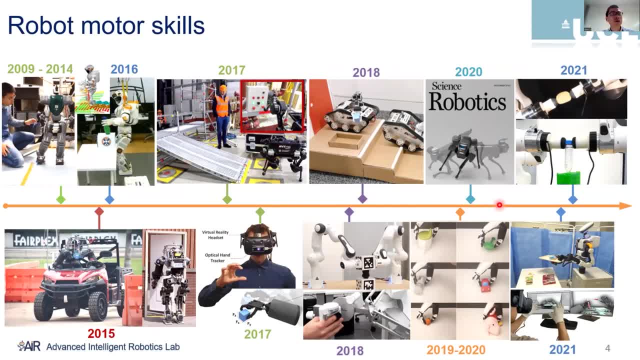 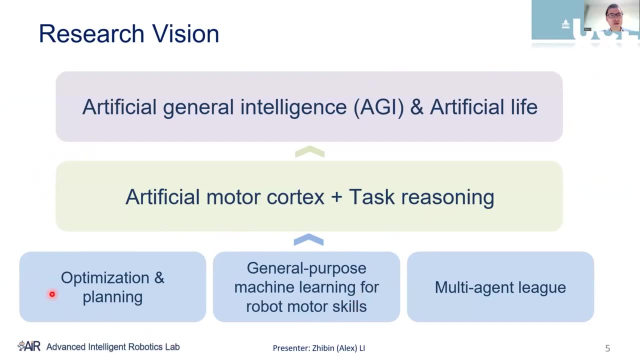 And particularly, I'm also looking for viable means how we can combine learning and control optimization similar to AI. So I'm going to move to what Ruben and Takahiro have discussed just now. So at the moment, most of the talks we have seen so far are staying on this stage in terms of learning optimization. 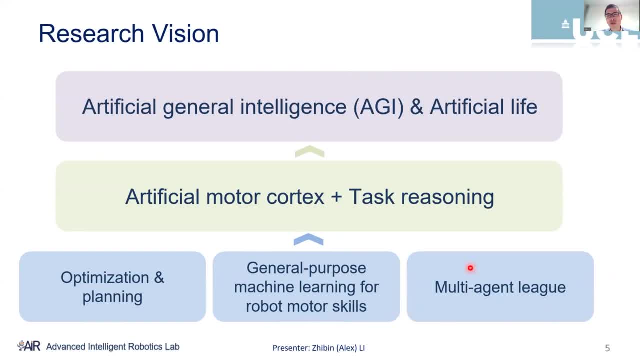 And personally I think, in long term, at some stage we need to move to the multi-agent way of learning as well. This will contribute to the artificial motor cortex And then eventually, I think, the overarching goal for most of us sitting here today. 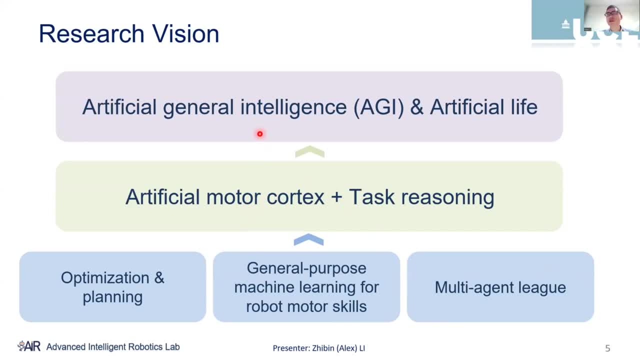 is to solve the artificial intelligence problem and create artificial lives. And personally, to me, if I would be able to reach the stage of making artificial motor cortex becoming true, it's already a great achievement before my retirement. So I'll quickly show the state of the art, as I have promised. 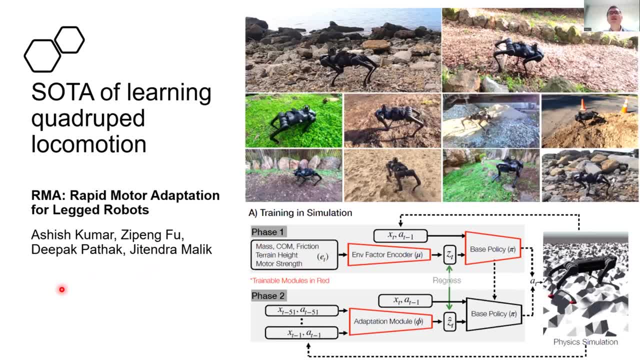 There are a lot of great works we have seen throughout this week. particularly due to limited time, I can only briefly go through three representative works here. One is the AMA paper. Particularly, there's a trend now that we use privilege information in the simulation. 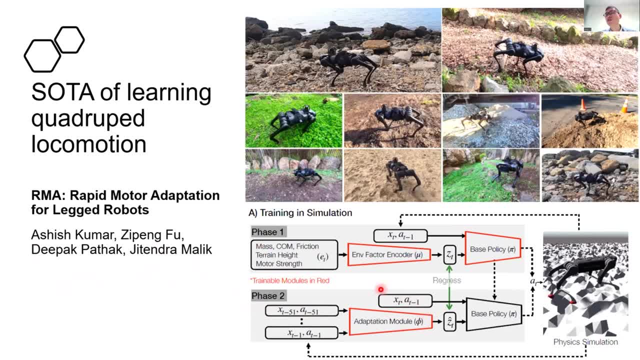 and then to train how to use supervised learning to train and extract the latent vector. Let's see how we can generate the efficient feature embedding such that we can use this low-dimensional data To train and learn the policy. So this is a very effective way of dimensional reduction. 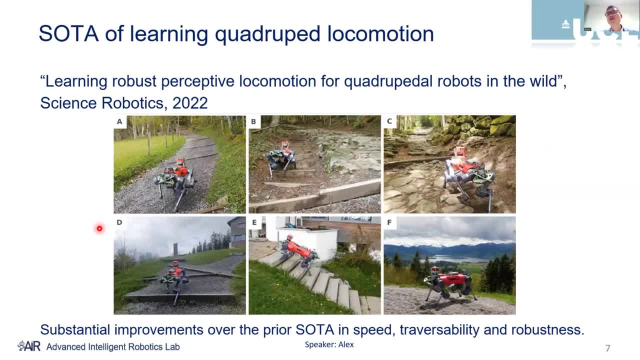 as you have seen from the previous talk, that using such privilege information, it's very, very robust to improve compared to the previous work. we have seen in the state of art in terms of speed, the versatility and the sector. So, with that said, there's also another work. 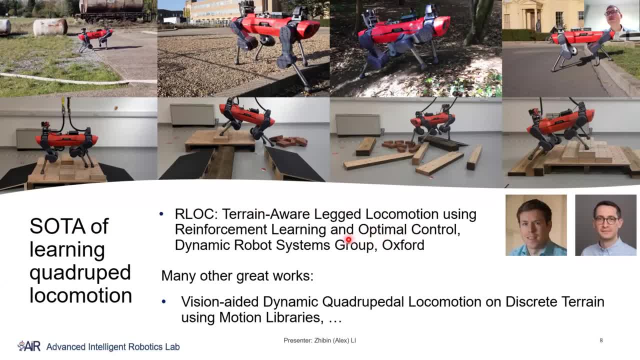 which tries to combine, try to bridge the organization and reinforcement learning as well. Due to limited time, there are a lot of other state of art I could not cover So particularly. I tri-picked those which are highly relevant to the talk today. 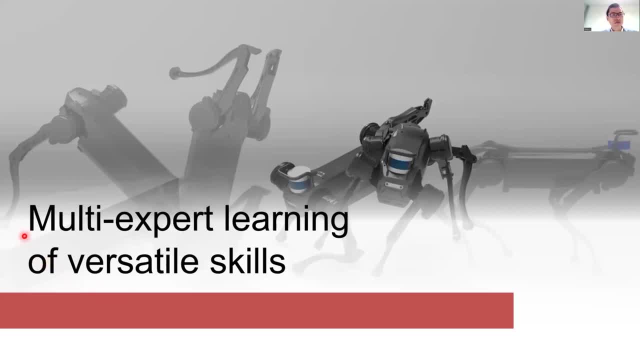 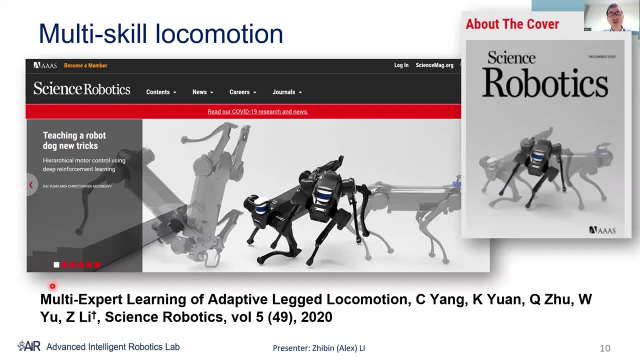 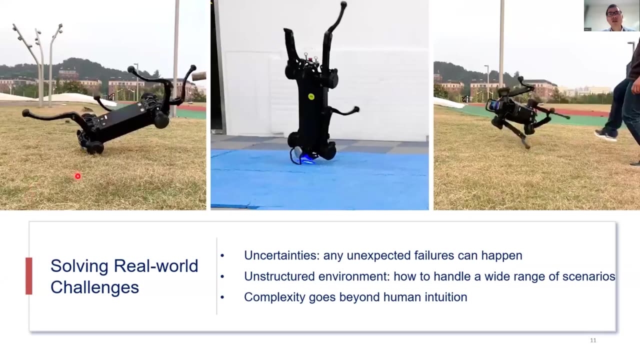 So here is the first of the three research trends I would like to cover in terms of the multi-skilled learning which is featured as covered in the 2020 report. So particularly this work originally is largely inspired by humanoid research, coming from my background- not quadruped- 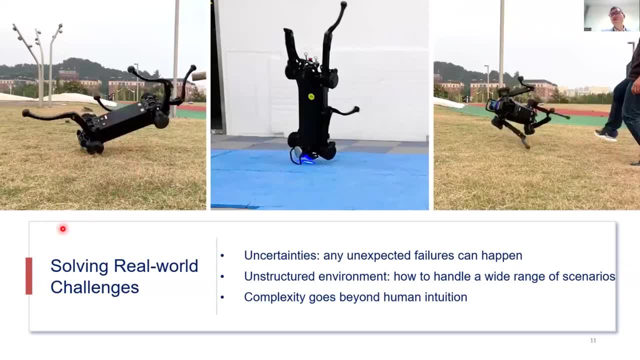 because original thought is that the humanoid robot should be able to walk, do all sorts of parkour, manipulate, dribble in the ball, play soccer, etc. And therefore it's very, very, very hard to use one policy that can do all the sorts of things. 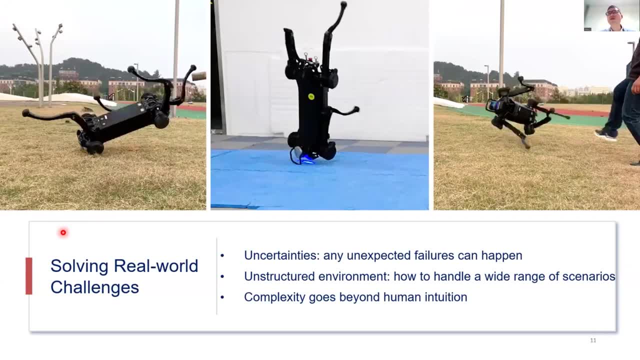 That's inspired the research of using multiple-hour policies and what are the viable means to train multi-skilled motors, multi-skilled locomotion, for example. So, particularly if we look at quadruped locomotion, this is all the real footage that has taken from the real-world experiments. 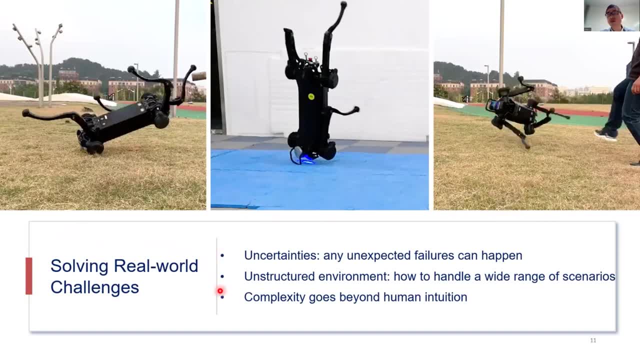 And the one thing I have observed is that, despite we can randomize a lot of cases, add a lot of disturbance in simulation, there's still a lot of cases in the real world that is very, very hard to simulate. We can observe something similar, but not quite the same. 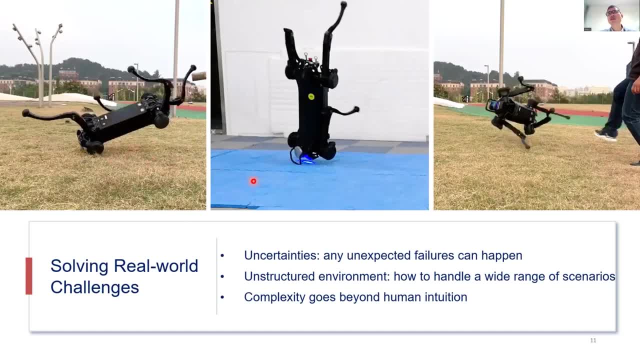 And, for example, the grass, the muddy ground of the rain and the slipperiness of the soft mat, and the robot can spin actually around. the gravity factor can spin around the vertical axis. A lot of those phenomenons are very difficult to observe in simulation. 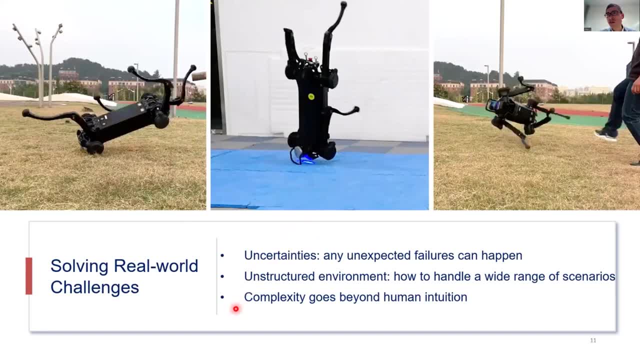 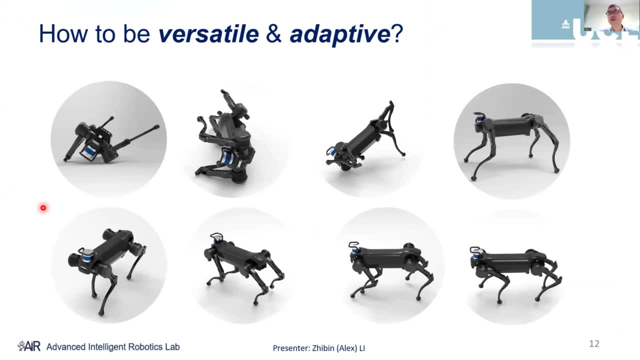 So, apart from the existing randomization techniques, that inspires a particular work, that how about the IR policy? If you look at single policy, usually we have a lot of existing techniques that can train you really really well to do one particular type of task. 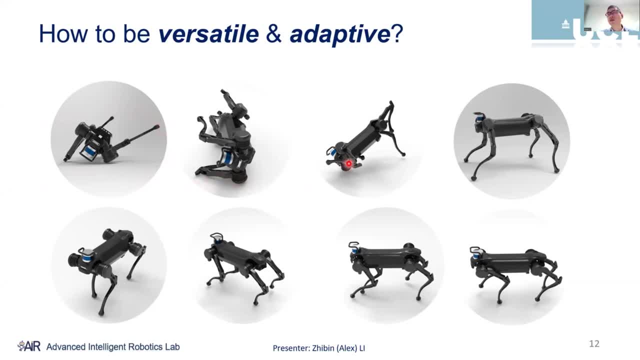 For example, fall recovery or rolling over the ground, and how it can fall and get up, how it can sprawl its leg, resist external disturbances, how it can quickly spin on the ground in a very gymnastic way, how to do trotting, galloping, bounding, pacing. 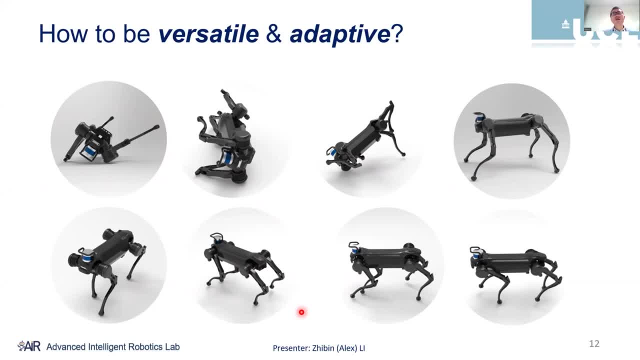 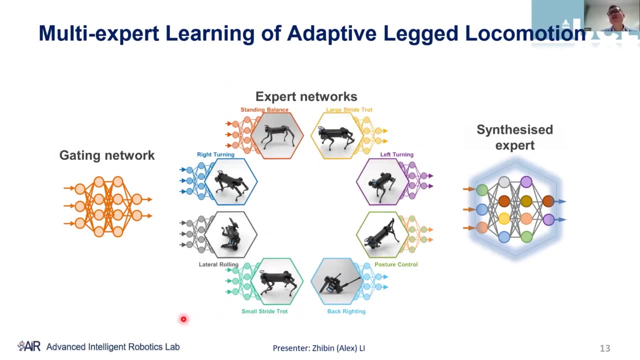 all different types of gait. So if we look at one particular IR policy or, let's say, a neural network policy, it's not hard to achieve such performance. So the question is that how we can bring all this in one bound to group all these capabilities. 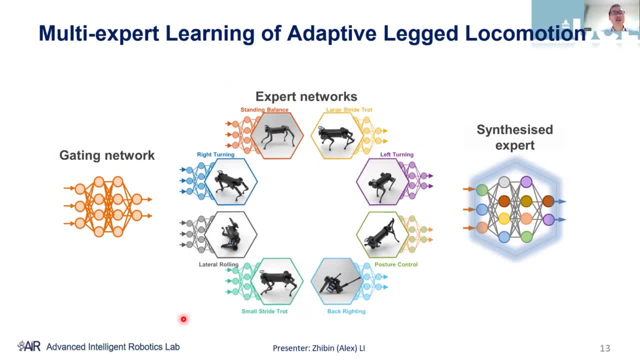 such that one robot is able to perform all of that. So that boils down to the thought that how about an hierarchical structure? So that inspires the work of MILA. so the multi-expert learning structure we have proposed in the science robotic paper. 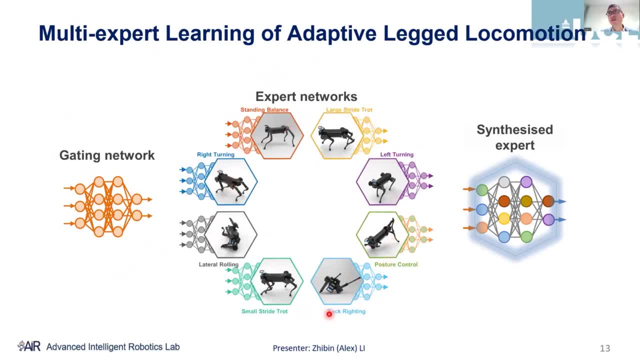 such that we have separate neural networks. For example, here we have eight experts. each is good at one particular type of skill- motor skill- And on top of that there's a gaiting network. here we can consider- let's call it- a coach. 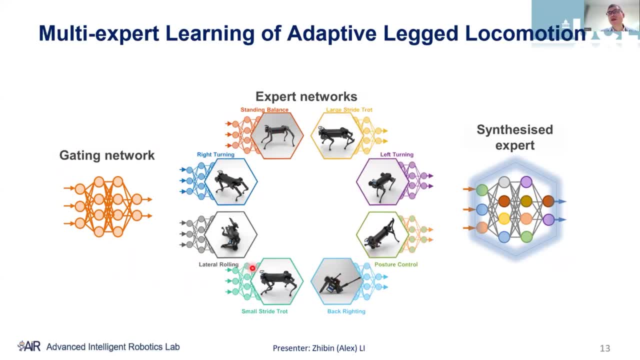 that can coordinate different players here. So the story here is that at different times different expert is needed for that particular situation and the gaiting network would activate that expert, or at different times different ones will be activated differently and such that we can synthesize all these experts. 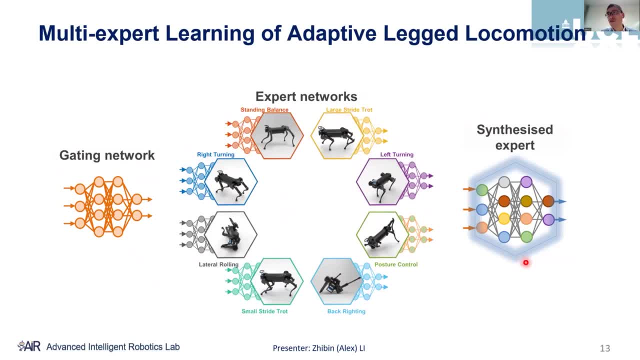 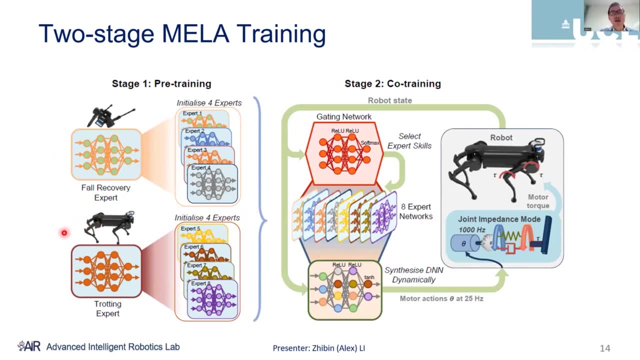 all these eight different experts into a synthesized one. We can fuse them together as one, such that they will be able to do cover a wide range of different skills. So, due to limited time, I will stay in the conceptual level that roughly speaking. 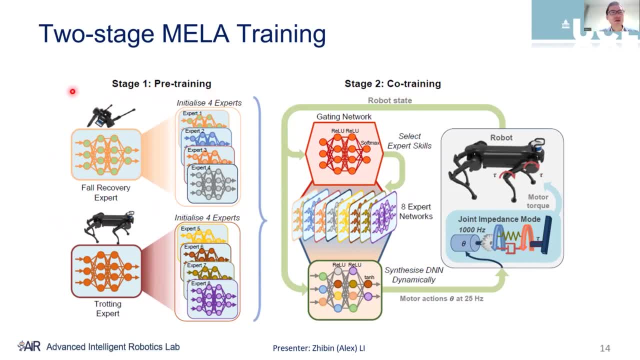 it has two training stages. It's very similar to a lot of topics we have seen before. Very often we boil things down into two stages. So first stage is that we will train very distinct skills first, such as fall recovery and trotting. 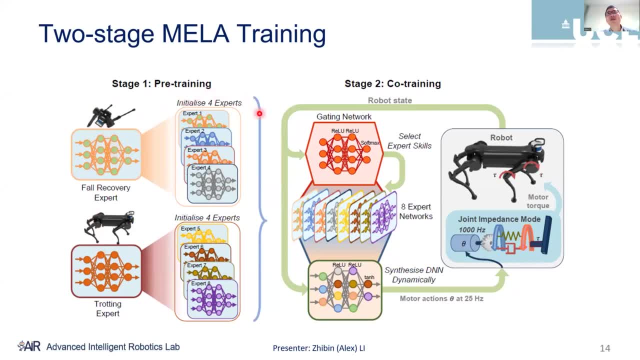 So these policies will be warm start policy to initialize other experts. So do not. it's the kind of rule of thumb that all the experts will get started from something. So here, where you equally divide them into two groups, initialize them And then after training that. 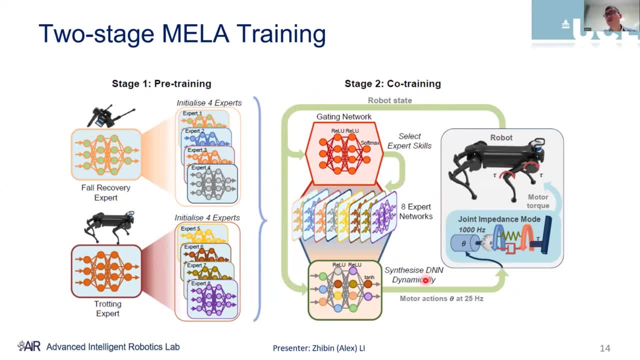 we come at the second stage to co-train them all together. So the takeaway message here, to make it easier to understand, you can imagine: this is the coach and we have eight players And after learning how to dribble the ball, pass the ball and strike the ball. 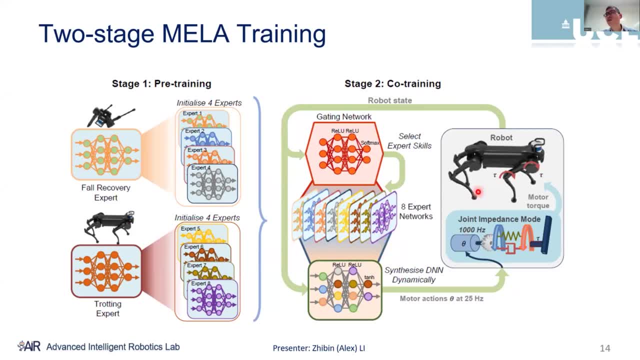 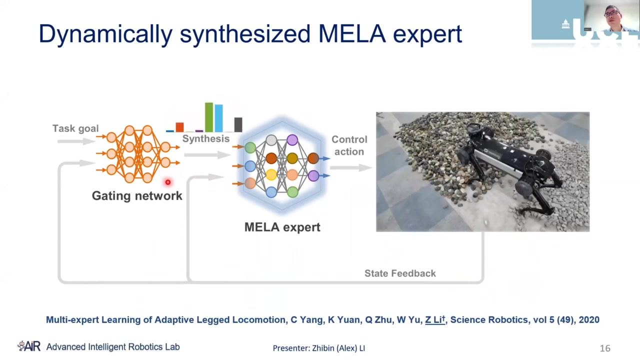 and all the players come together to train in different simulation scenarios, right? So the rest of the setting is pretty standard. Impedance control for the talk to robot, because in simulation we have perfect talk source. So here is just a visualization which matches the classical feedback control. 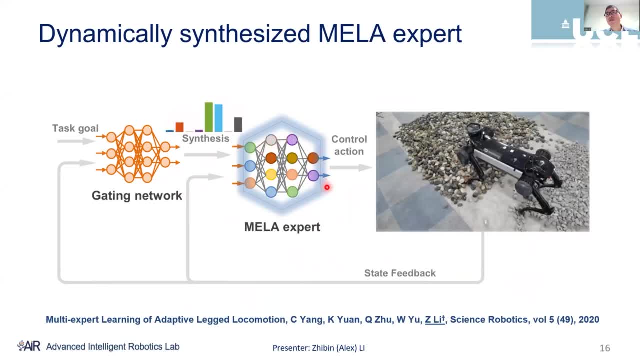 So we have a dual loop here. The synthesized expert is taking all the state feedback here, which is probably the pre-accepted feedback, And the gating network will see the same observation, plus the high level task goals in order to activate all different experts. 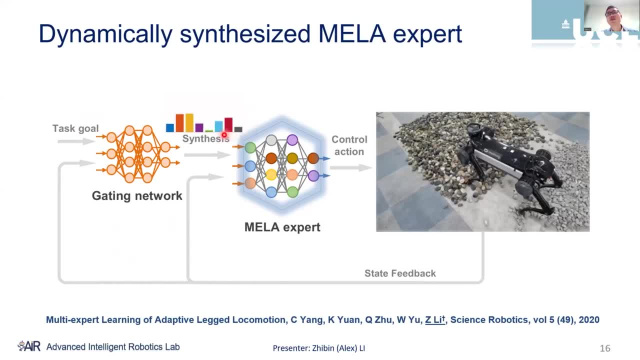 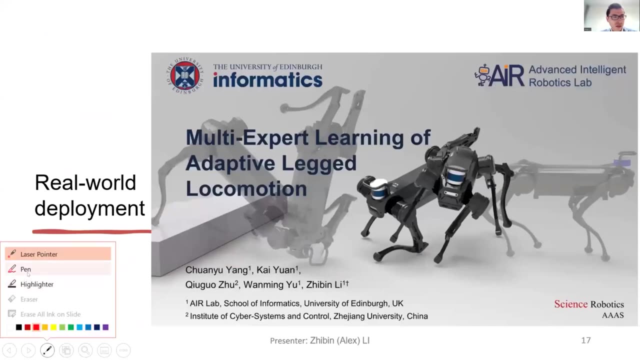 So, as you can see here. so the different expert is illustrated with different color and it's pretty much like a music bar, right? So all of them coordinate and get activated in harmony according to the situation. So here I will play back very quickly. 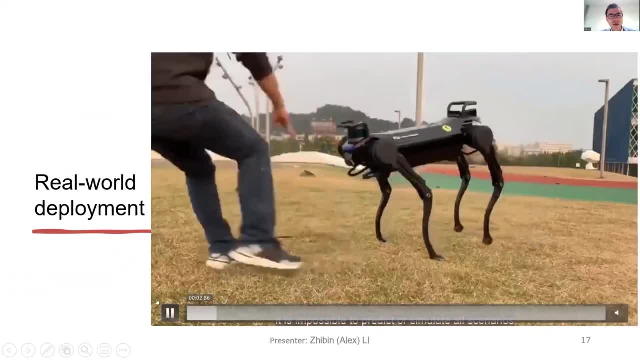 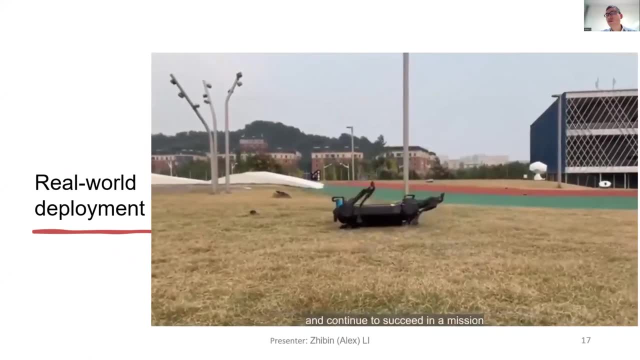 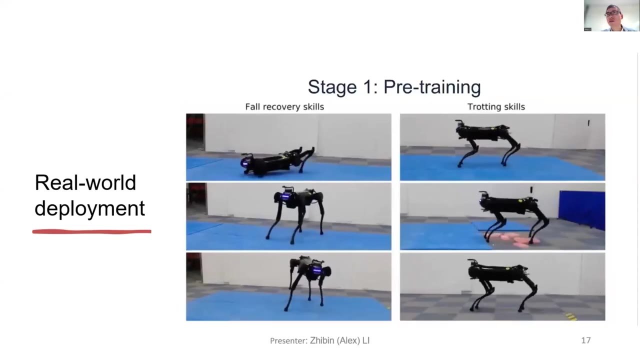 the key part of the video. So this is the full recovery that has been trained before and the robot can, so we didn't apply any domain randomization and it works right away in the hardware. And this is how the full recovery and trotting works. 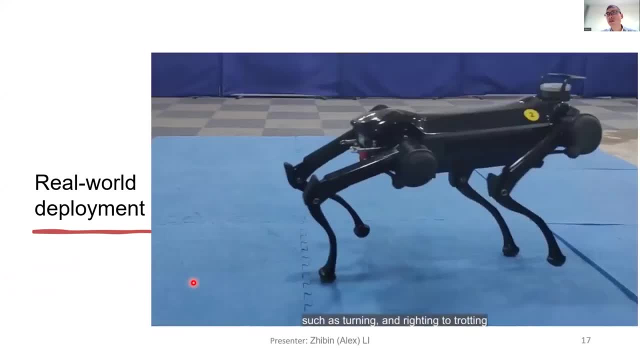 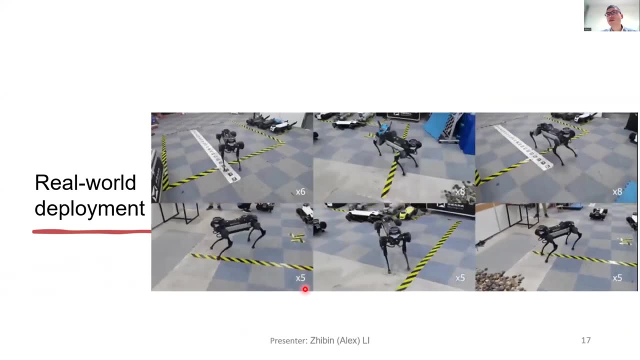 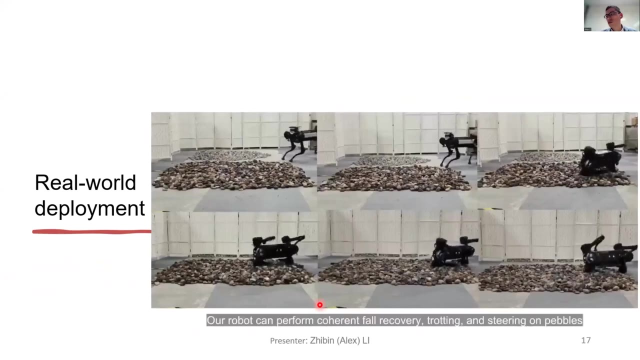 And it also extrapolates some other skills. So, as you can see here, by fusing different neural networks together, so the full recovery and getting up there are naturally combined. So the fusion allows all these different policies to figure out their own transitions. 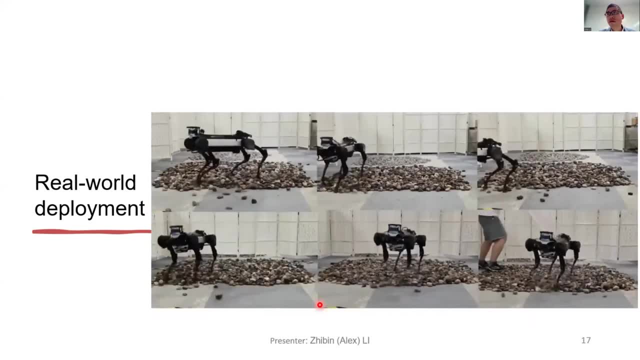 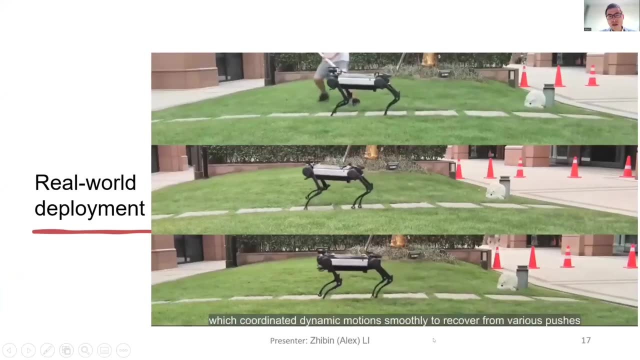 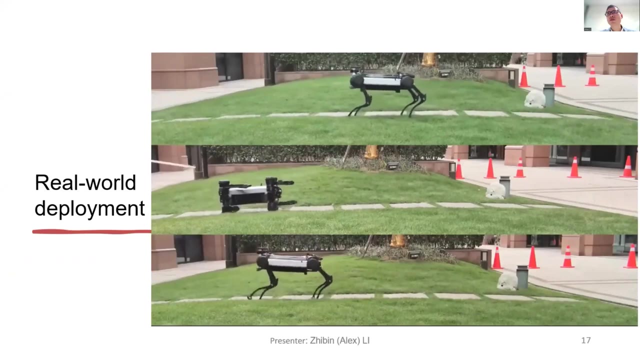 So we don't have to hard code. All right, So let me skip this part. So, as you can see here, the full recovery will be continued. if the robot doesn't recover once, it can continue doing so until it succeeds. then continue trotting. 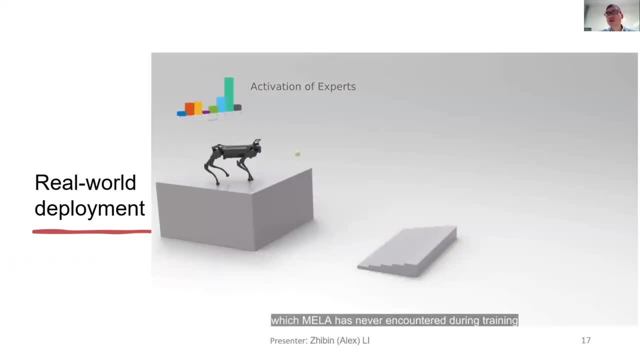 So, in particular, there's more detail we can see from simulation. We can do a crash test like this, which we cannot do in reality. So here's blind, There's no vision, here It's purely blind walking. So particularly I really like this moment. 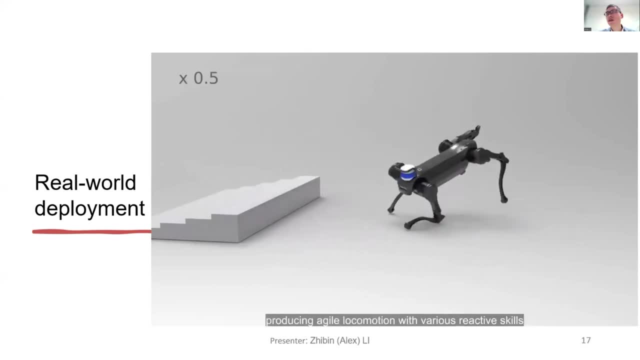 You can see how the legs coordinated according to different state feedback and the robot can spin very, very nicely. So let's see it again. So you can see how the retrieves the leg avoid collision And when spin on the spot and try to turn as fast as possible. 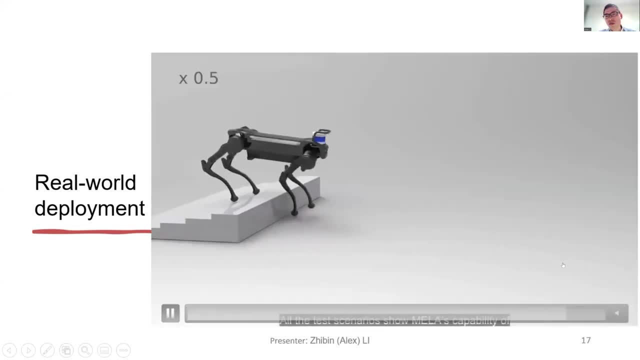 it actually uses three legs rather than four legs to have very, very small friction, So it can spin on the ground very, very quickly and then resume the gate once the heading is right. So all of this we find it very, very hard to do. 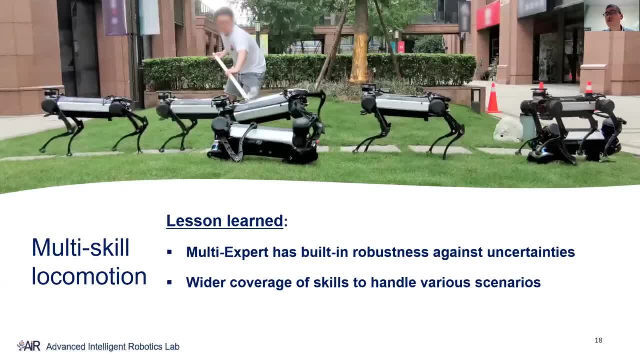 It's very hard to hard code using traditional optimization, parameter optimization method. It's very hard to parameterize these features. There are a lot of lesson takeaway messages, but two key points I'm happy to share here is that we found out interestingly. 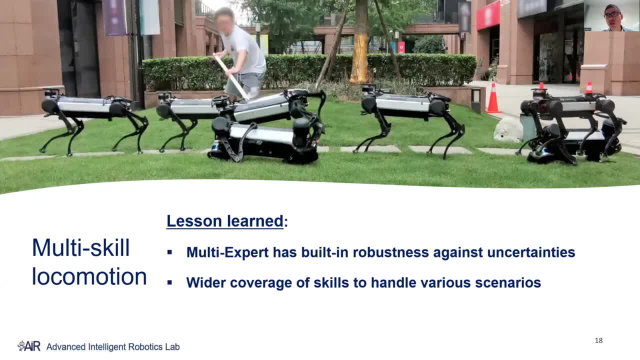 because there are a lot of experts within the whole integrated structure. we find that it's quite robust because different experts can act in the right time, even when some things are not seen before. they're quite robust against those uncertainties And also particularly if we know. 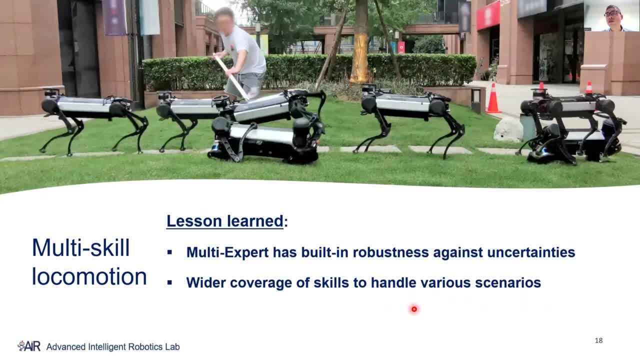 there are a wide range of scenarios and this scenario is very different from each other And this framework is much easier to train and is much easier to alter compared to the traditional way, if we just do anything through one single neural network. A small question here is that 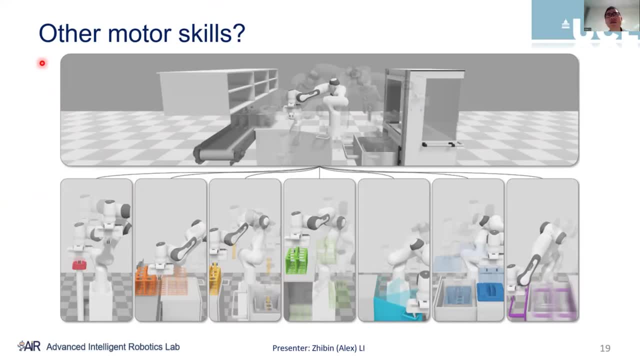 how about manipulation? I got asked very often about this. The short answer is yes. it's a positive answer that the similar scheme can also be used to have different manipulation skills, as you can briefly see here through snapshots And the robots using this multi-scale framework. 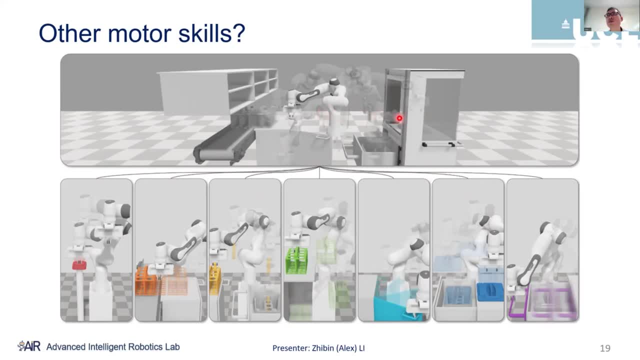 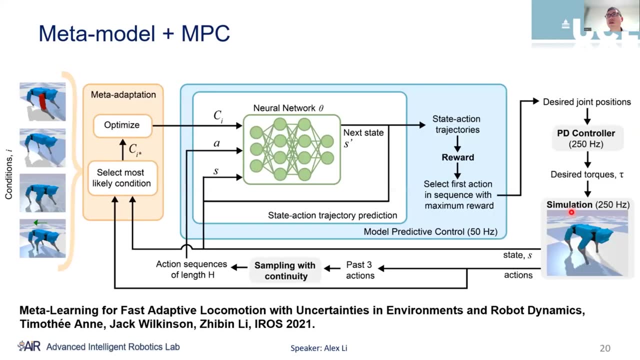 is able to operate along horizon a sequential and long-horizontal scale, And so we can see that there's a lot of manipulation tasks in the long-horizontal scale. Okay, so, very briefly, as we have had a discussion about model-based versus model-free, 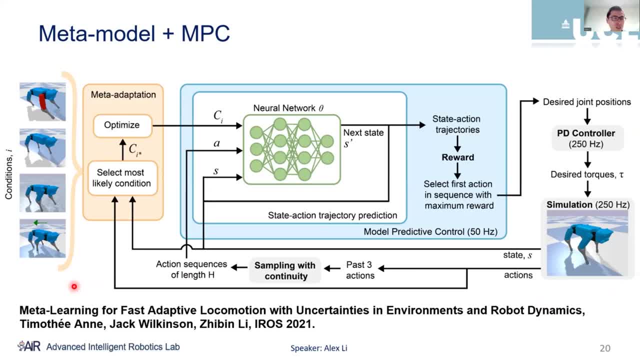 or like MPC versus IO. I'd like to quickly share a small student project that has been done last year, like two years ago, and published last year in the IWAS. So we find out that there are different types of tasks that can be used to train one network. 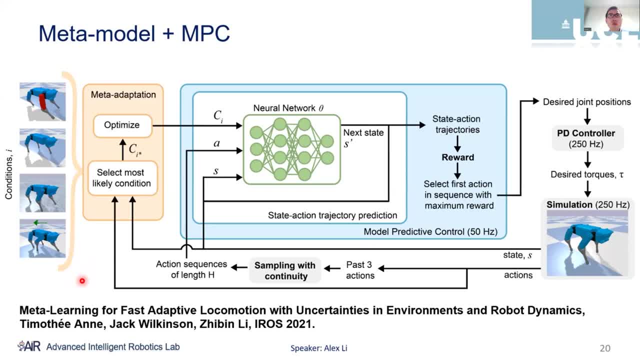 And, as I said in the beginning, we are able to train one network super well to deal with one type of task when the modality of the configuration does not change. So maybe there are some corner cases that learning cannot cover, But in most cases 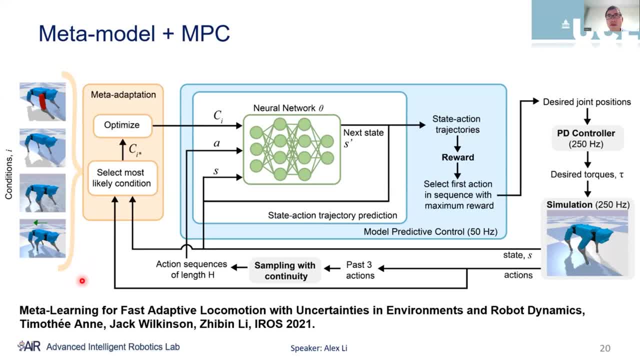 as you can see, usually when we test outside, it doesn't fail that badly. But, however, when the modality of the configuration operation changes a lot, If I block one mode and one mode is jammed, or if I cut off one leg of the robot, 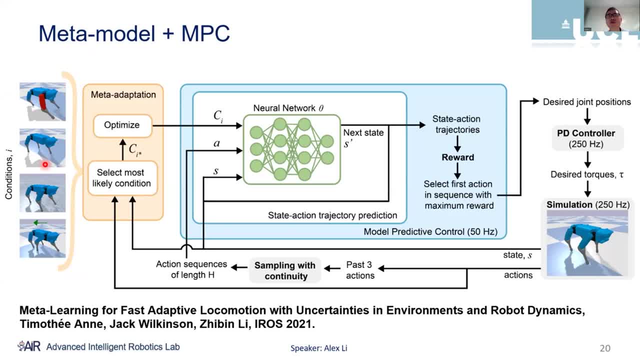 so I believe many of those policies will fail if they're trained in the single scale right. So if I just chop off one leg of the robots, that our policy has no way to work anymore. So that inspired a way. there's some discrete nature of the locomotion problem. 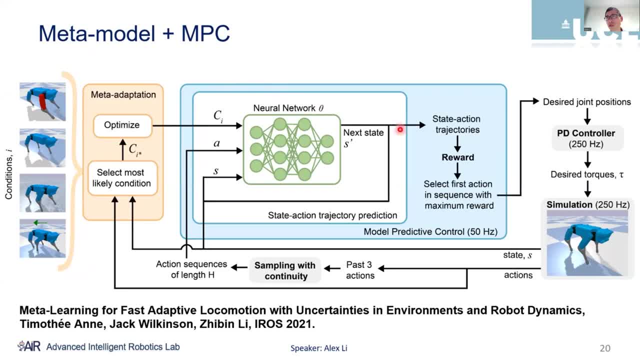 and continuous nature, And this we also have neural network as a functional universal function approximator that can do the job, And we also have MPC, which can exactly embed the constraints. So what is the nice way to put all these features together? 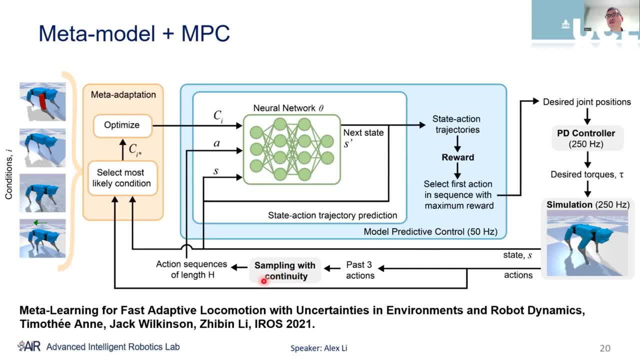 I don't have the final answer for that, but this interesting small student project shows that we can do it through by embedding the interaction model inside the MPC. So you have it here. different conditions: We have the feature embedding here that we only need to collect the past 10 samples. 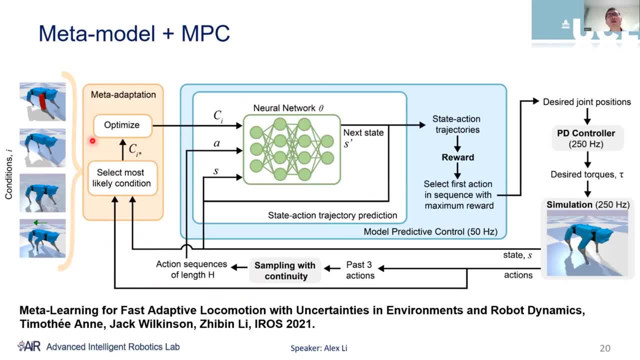 within, say, 0.2 second to understand and optimize, and try to understand what is the most likely condition now And using that condition, and then we can update a new network which represents the interaction model. So this is very, very similar. 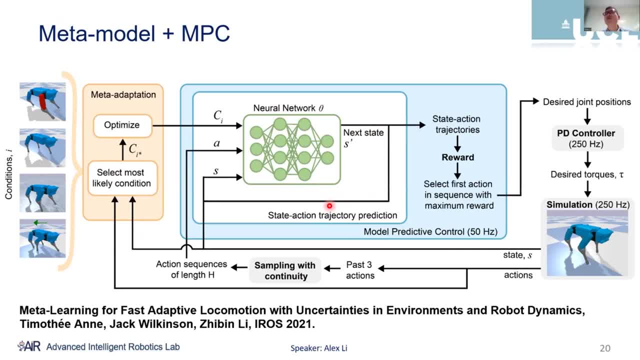 to the traditional model we use for MPC right, For example, simple single point mass model or the linear independent model et cetera. But instead of that we just use new network for the model. The rest of the MPC is quite straightforward. 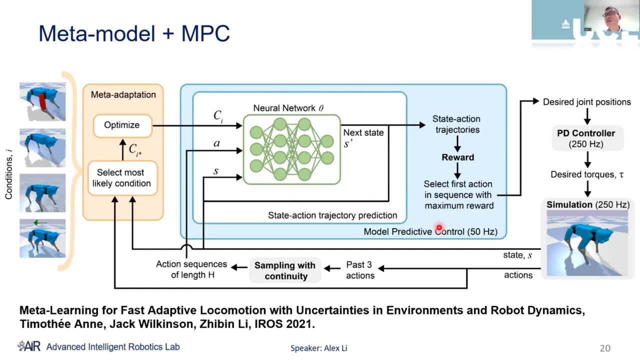 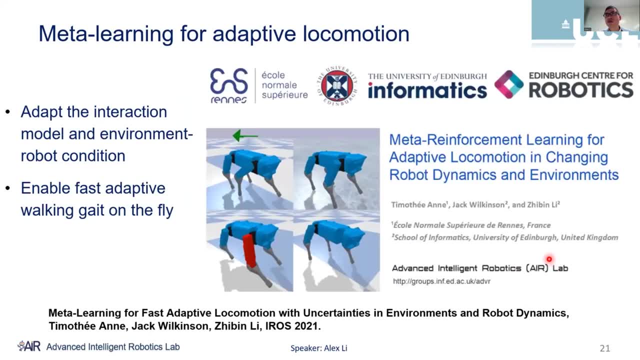 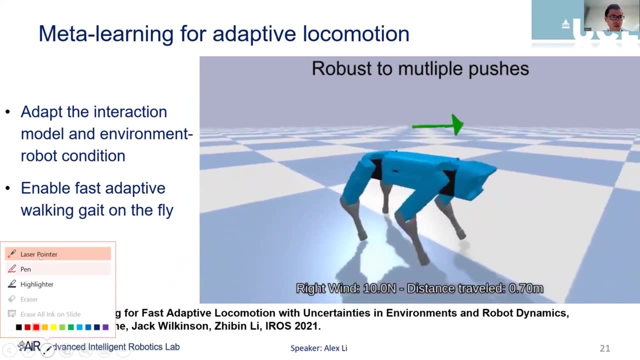 We can make it very simple. We can embed drawn limit, acceleration limit, a position limit, et cetera, And the beauty of that is that the nonlinear features of the interaction can be captured very well. And let me speed up a bit. 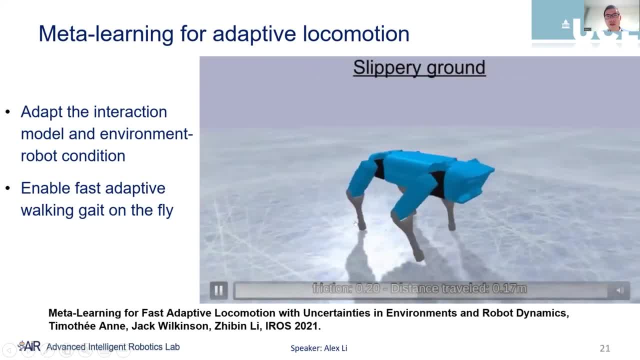 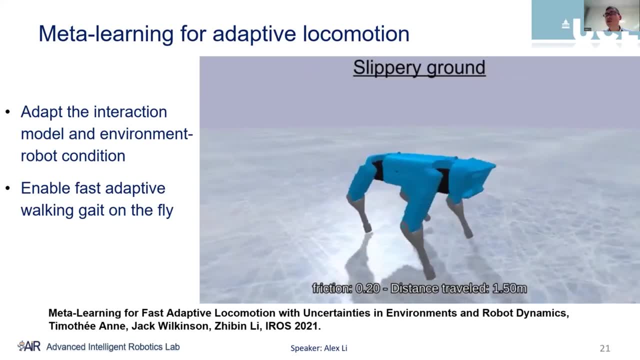 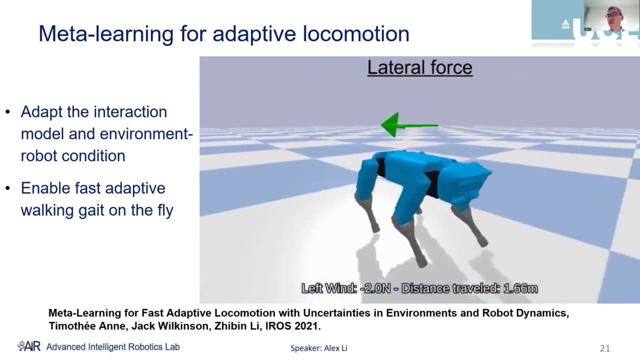 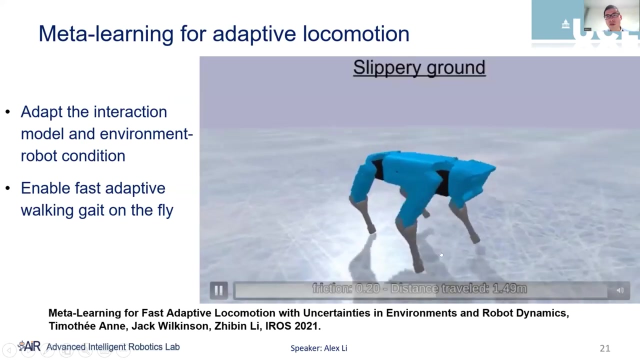 somewhere from middle. So we can. so the new network can fit very well. the nonlinear interaction model with the environment And the MPC is good at figuring out how I can, how the robot should act in order to counterbalance these changes. So for example- sorry, let me do it again- 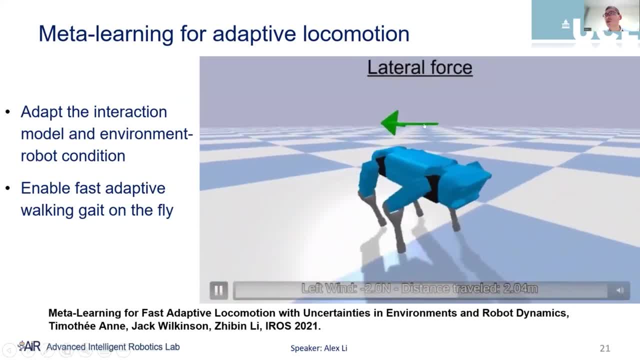 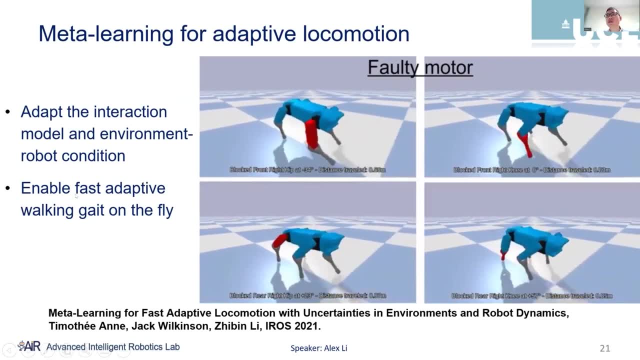 So, for example, here you have a continuous external push, So the interaction model knows that there's external push and MPC can figure out what is the best way to do that to counterbalance the external perturbation without changing the heading. And the same works for 14 months. 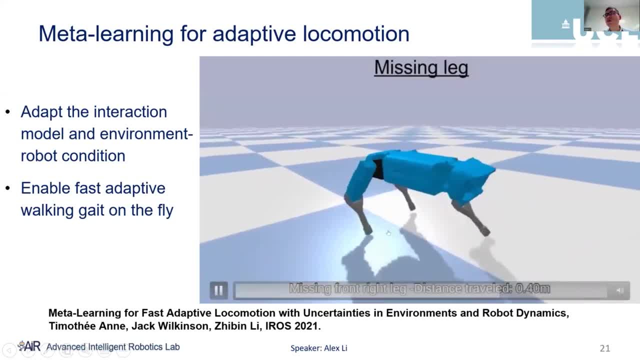 You can jam one motor here at different places, or you can even chop off one leg and the robot can still walk. So the MPC can figure out, given all the joint constraints- accelerate constraint, velocity constraint, et cetera- now the interaction model changes. 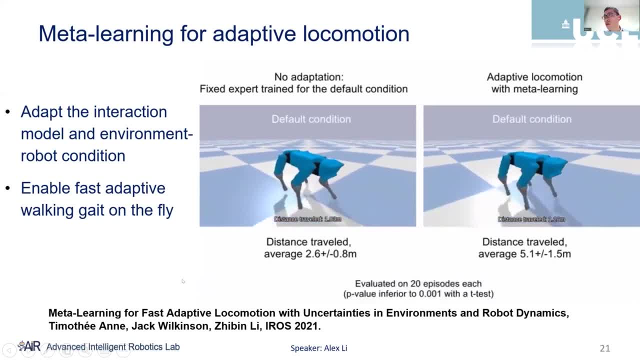 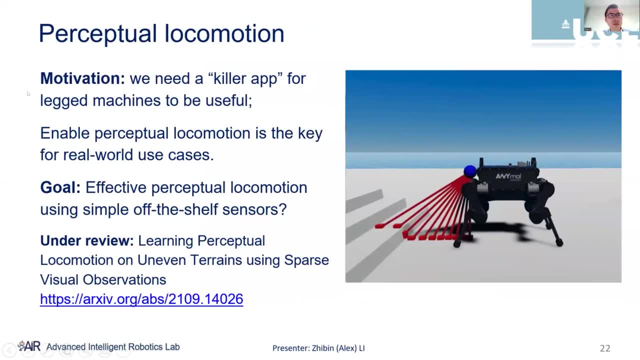 and what it should do in order to sustain the working velocity. So that's just about the meta-learning part And, interestingly, I would like to share a work about perceptible data. So I'm going to show you an example of this. 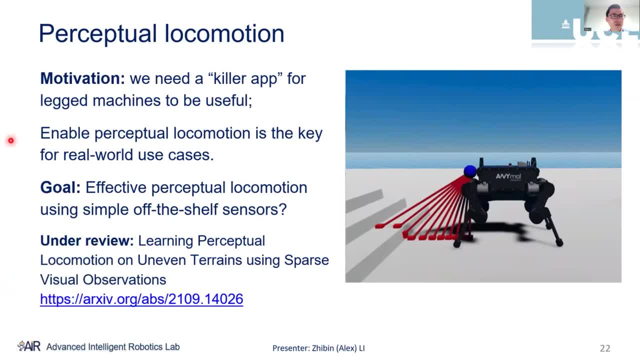 A perceptible locomotion which looks at the problem slightly from different angle, And I think I have to answer from answer for Tadahiu's question before how in terms of the naive solution. So here particularly we are thinking about how to find a killer application. 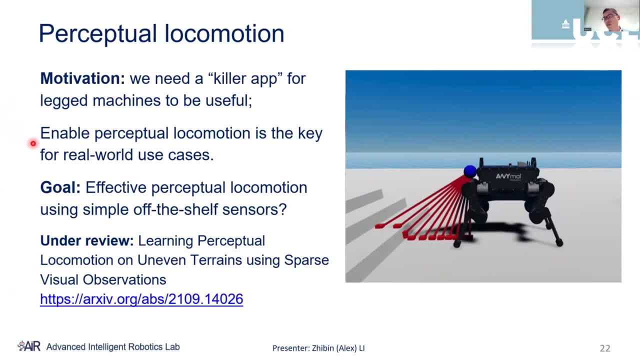 for, like the machines, to be useful, So in this case it needs to be very, very easy, simple and low cost, And, in order to be widely used, it needs to be very, very, very, very, very low cost. 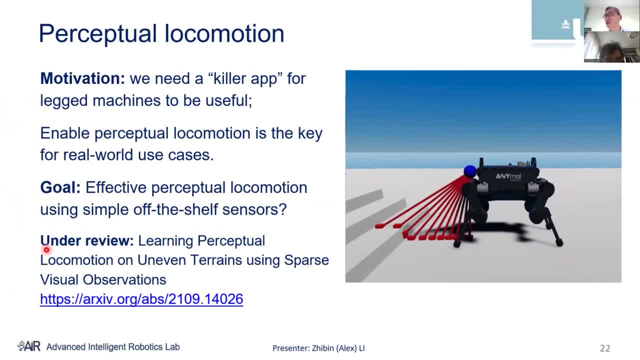 So the motivation is that what is the simple way to do? and we have current paper that is on the review And we found out actually there is a way to directly put the height map effectively in this representation. here it's represented in terms of rays in the polar coordinate. 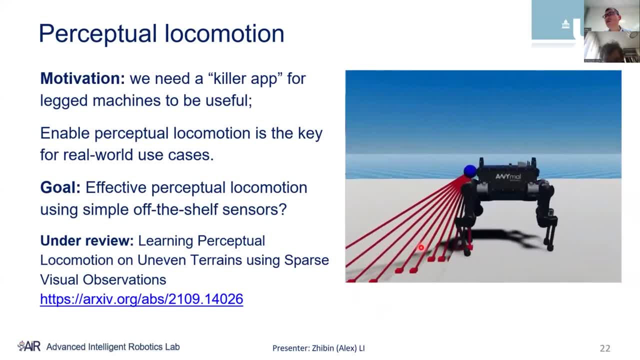 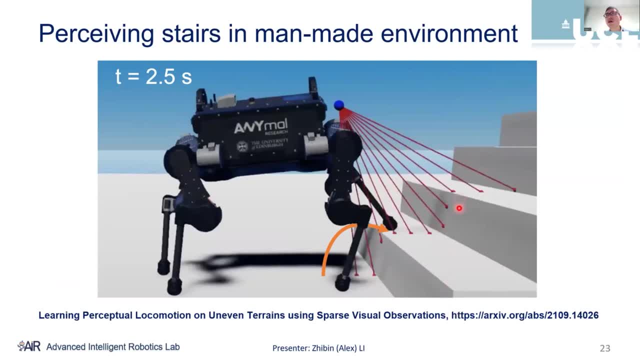 However, I should point out that it's a very specific case. We look at very, very specific types of stair-like terrains in manmade environment. So the reason is that, as I mentioned, we look at the killer app. So if you look around our environment, 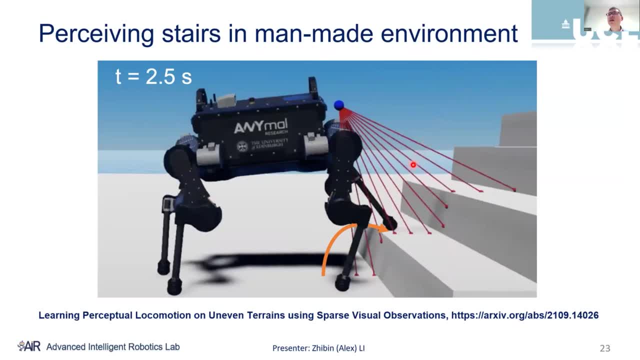 mostly it's flat planes and the only place we need legs to negotiate is basically stairs, right Or stair-like a step. So in that case it's a very, very particular type of terrain and we only need very few and sparse visual observation. 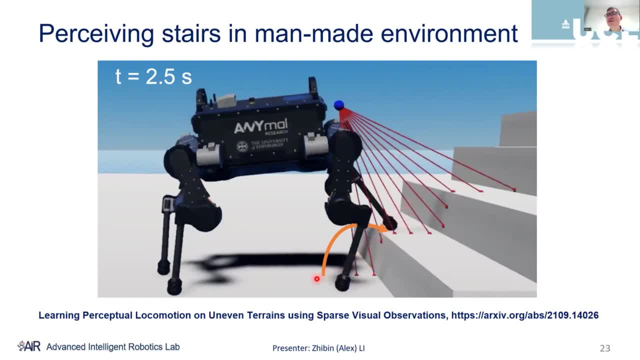 in order to capture this profile And such that we figure out within the leg workspace here what is the best action that can negotiate this terrain height right, So this terrain height can be captured by the ray length here. So in this very, very specific application, 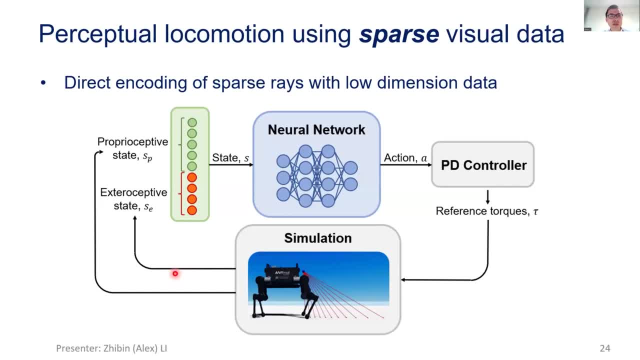 within our daily environment. we do not need very complicated structure and therefore we can extremely simplify the structure and make it very, very cost-effective for the real-world implementation. As you can see here, it's a very, very it's a vanilla application here, right. 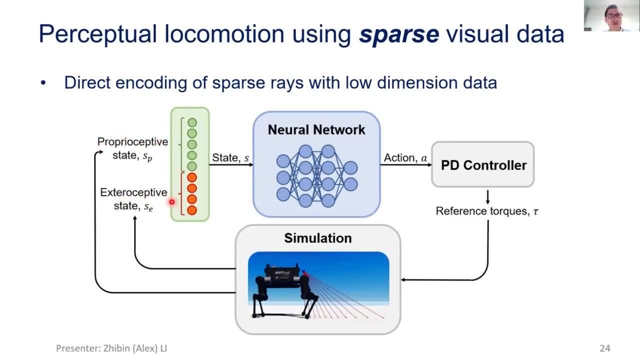 You have the proprioceptive information and extraceptive information, You would get feedback here and train it. So, as Takahiro has mentioned, if you simply put in this way, it's likely to fail. So particularly what the paper is about is: 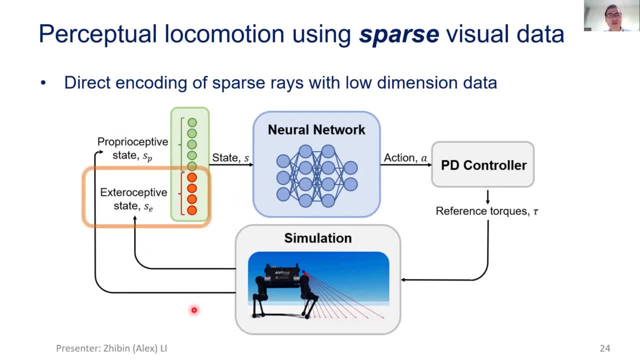 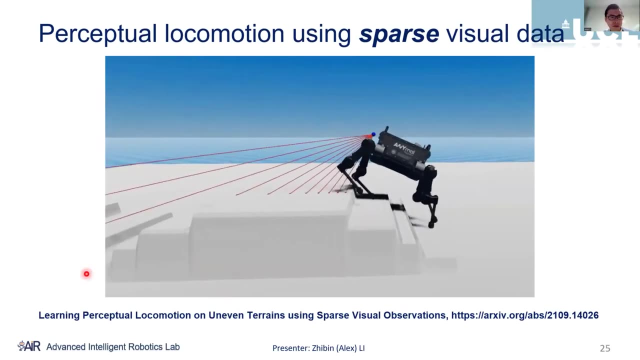 to offer a curriculum such that it's easier to learn a new net policy as such. So in this way, all the rest of information is easily available with most of the hardware. Okay, so I have three minutes left, So here's just to show that it can negotiate. 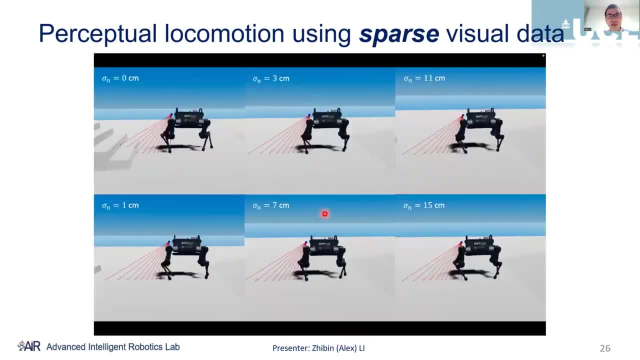 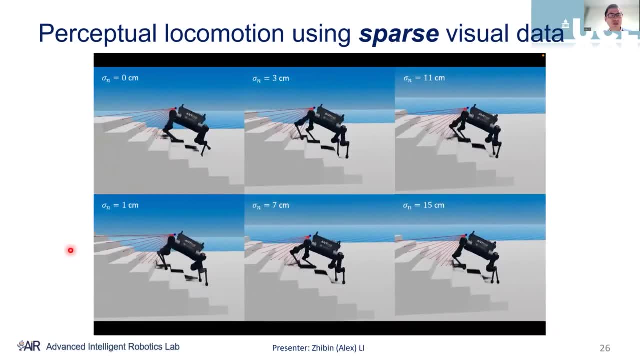 with most of different stair-like terrains in our daily life And we also put a lot of noise here. up to 15 centimeters standard deviation and it still works with stairs. So if we only look at how we can use lighting machines, 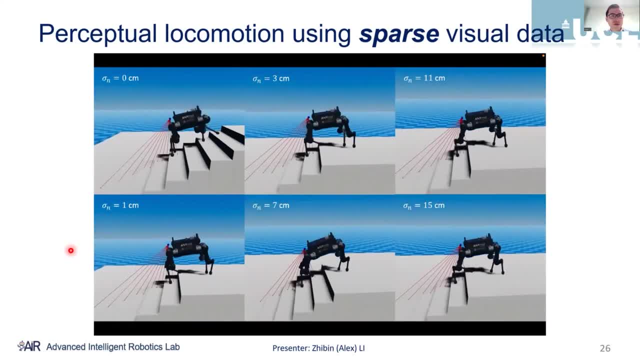 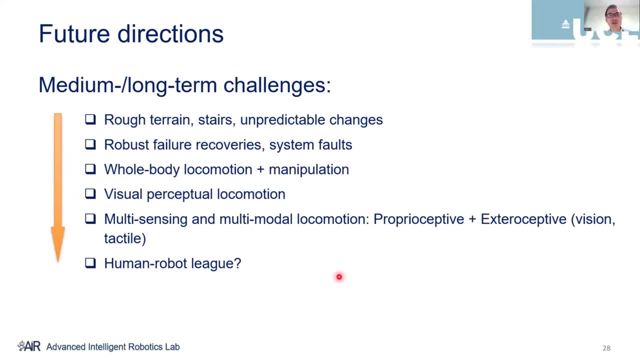 for daily environment, like stairs. we can see that the data is very, very low cost, cheap solutions Very quickly to talk about future work. So those are the topics you have seen throughout the week And I believe there are still media and long-term challenges we're going to solve. 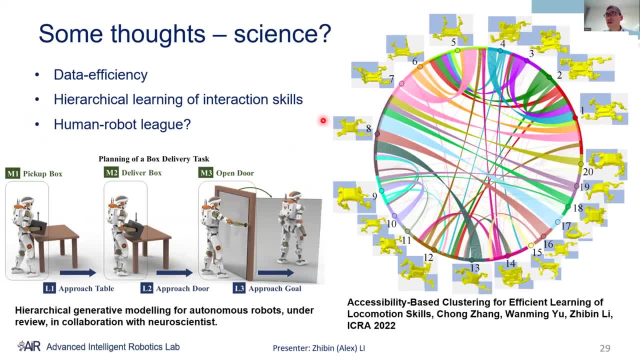 I in particular share some thoughts here is that the data efficiency is one of the problems we are looking at in the research group And there's a work about connectivity presented this week. So different configurations have different connectivity and transition between each other, as you can see here. 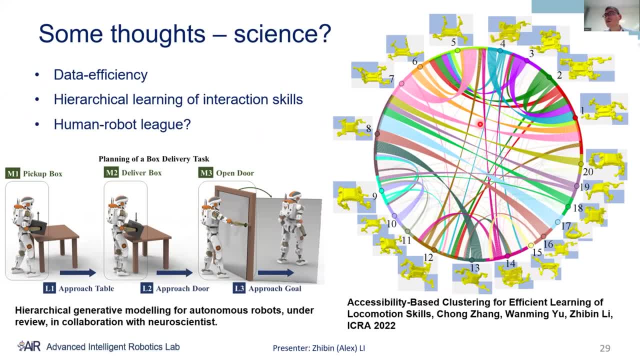 And the duality. the dual way transition has different level of difficulties. For example, falling down is easier, getting up is more difficult. And in this way we know what is the probability distribution between different states or configurations And therefore we don't have to do uniform sampling. 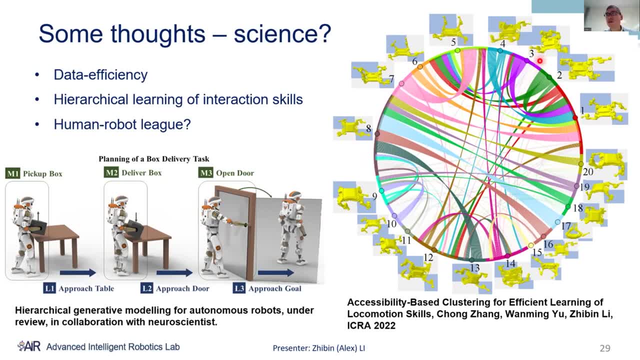 which is not data efficient right. So if we understand this better and then we can improve data efficiency. another point is the hierarchical structure that we can take some inspiration from nature. That's how we can design hierarchical structure. That's where we can put different learning or MPC. 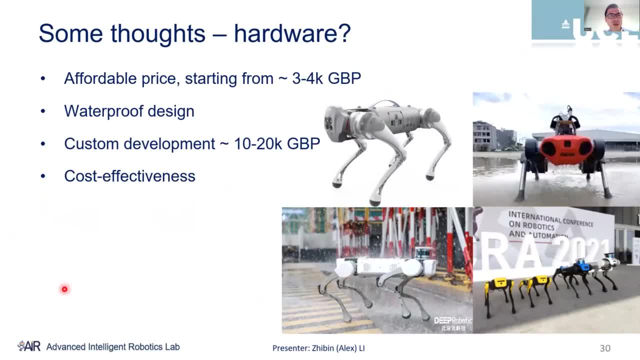 or different controllers into one framework. So another thought to share to inspire some question and answer, is that now all this hardware becomes so much available and the price is getting lower and lower. So the KDA app idea is that to put simple rates as such for stair climbing, that can be done. 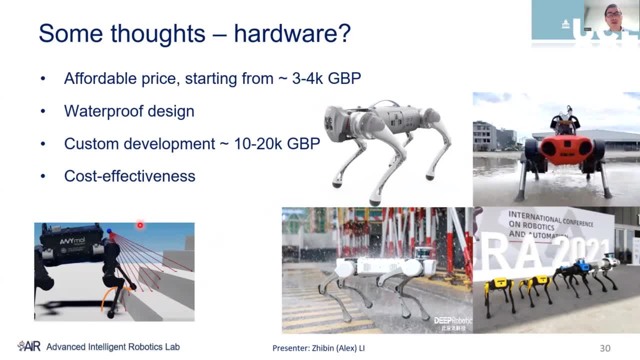 So the idea is that to put simple rates as such for stair climbing. that costs nothing And also the new network is relatively small and very easy to run. This means that if we can bring the cost further down, we will be able to see a lot of robots in real life use. 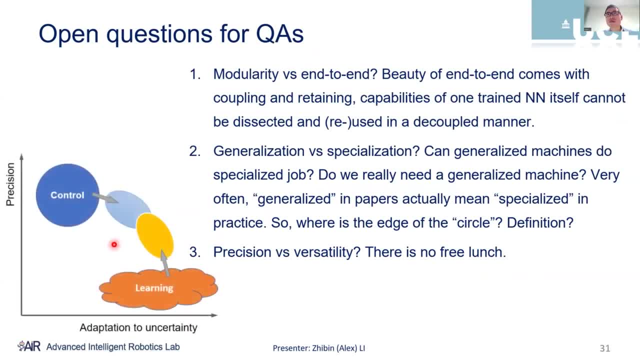 There's some open questions. I have written here. Some of that map to the previous session very, very well. Coincidentally, for example, control has a lot of precision, like what was mentioned before. in terms of MPC. you can precisely put foot over the stepping stone. 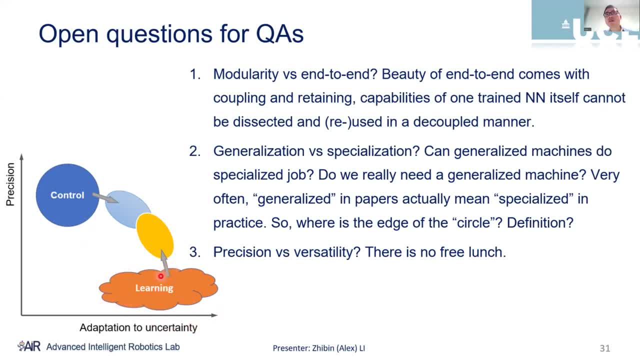 but learning has a lot of adaptation to uncertainties in the wild environment. So the learning uses the new network's probabilistic prediction of actions to maximize the reward and success rate, which works perfectly for the outdoor environment. Okay, so I would like to conclude my session. 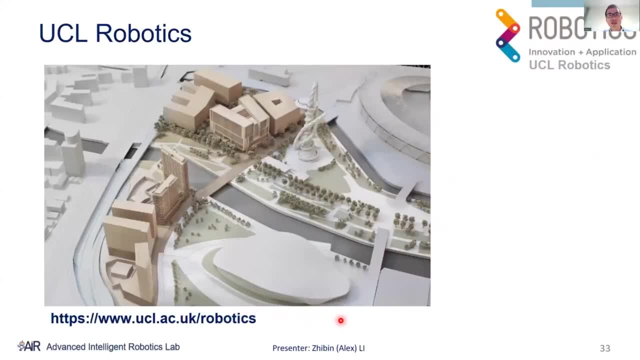 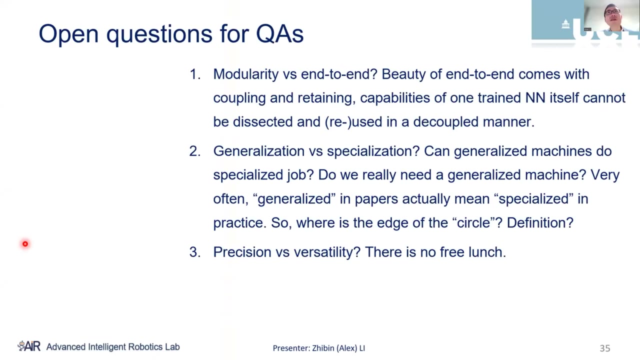 by. thank you for your attention And a short note is that UCL is expanding its robotics initiative in the Olympic Park And we'll be hiring, So I thank you very much for your attention And I will leave the question here for the discussion. 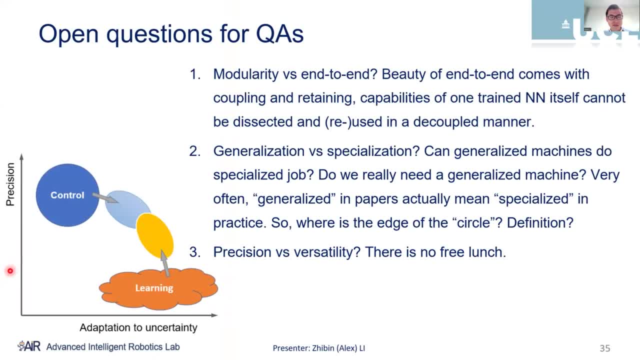 Are there any more questions or comments from the audience? I think we have to wrap up. We'll close the session off here And, if you have any, if you want to leave a comment, just let me know. I don't know. 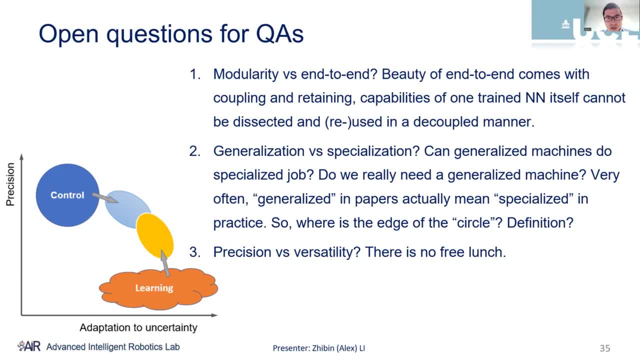 but just say hi there And I'm gonna answer your question. If you have any other questions, please feel free to let me know. Are there any more questions that you have, or? I hope not. So thank you so much for your time. 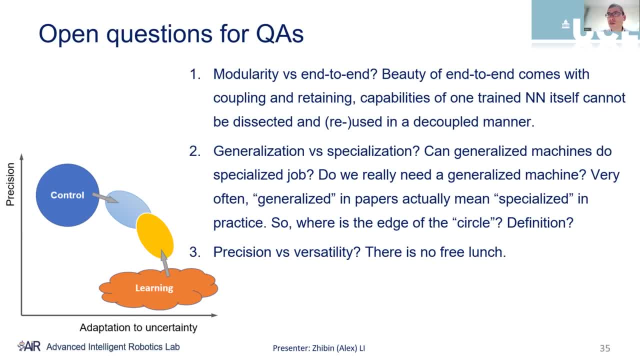 I'm going to say goodbye to Thanks and have a nice weekend. Thanks for the great presentation. Thank you everyone. My name is Xiao sings Nice. Thank you for listening. I appreciate your time today. Thank you all very much. to the stair without an angle, something like that.